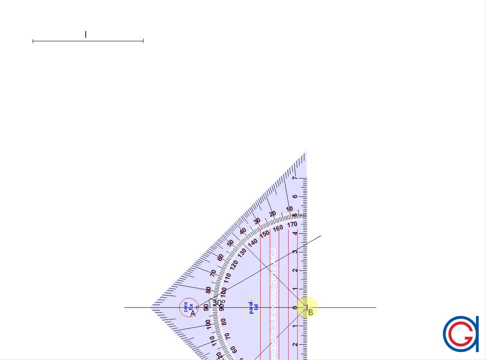 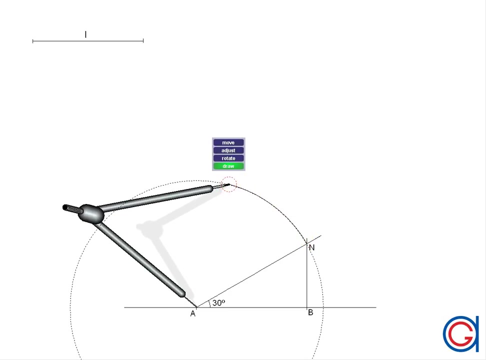 B, which will intersect our previously drawn 30 degree line at a point N, as can be seen here in the video. So the next step is setting our compass to the length AN. We scribe an arc to the left, as can be seen here. The next step is to draw the perpendicular bisector. 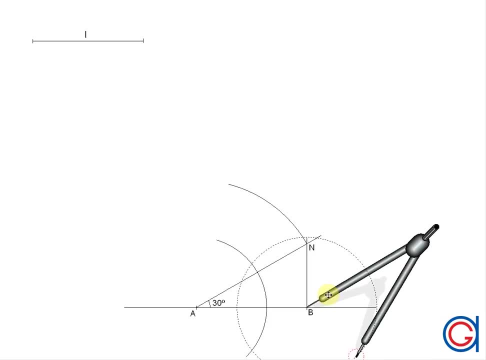 of the given length AB. To do this, I remind you, we must draw two arcs with the same radiuses. These radiuses must be longer than half of the base, as shown in the video. And now we will draw the first arc with the compass centred on point A, and then a second arc with 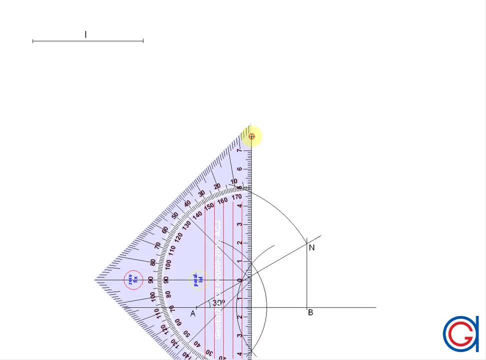 the compass centred on point B. These arcs will cut each other, above and below the line. The perpendicular bisector is the line which passes through these two points, And this perpendicular bisector is going to intersect our previously drawn arc at a point which. 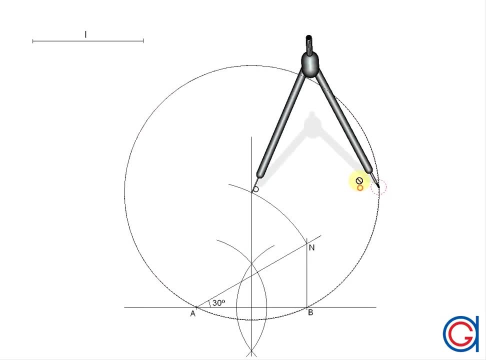 we call O, And this point O is going to be the centre point of the circle that we are going to inscribe our heptagon. So now we are going to draw the circle, As can be seen here in the video. Now the next step is setting our compass to the length AB. We are going to scribe six. 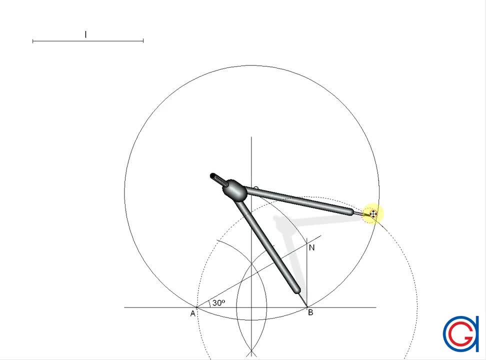 arcs around the circumference. So here, setting our compass on point B, we scribe our first arc And now, setting our compass on the previously drawn arc, we scribe our second arc. Again, setting our compass on our previously scribed arc, we draw our third arc. 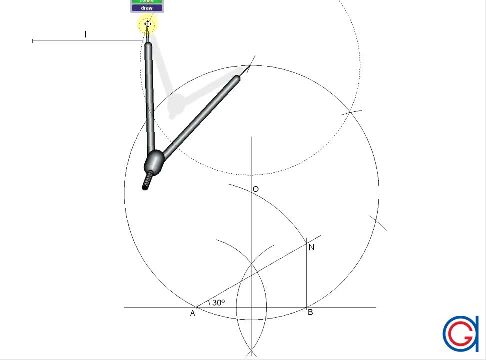 Again setting our compass on our previously drawn arc. we scribe our fourth arc And now our fifth, And if we have been working with precision and accuracy, our final sixth arc should cut exactly with point A, as can be seen here. 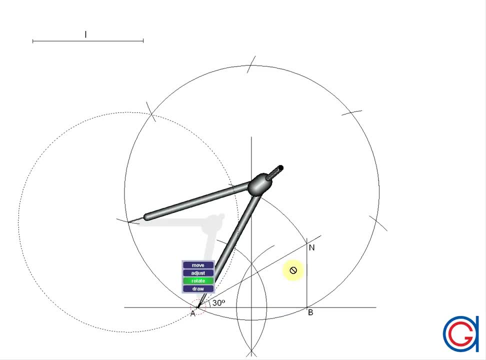 So it cuts exactly with point A. This tells us that we have been working with accuracy, And the next step now is to name all of our new arcs or vertices, So A, B, C, D, E, F and G.